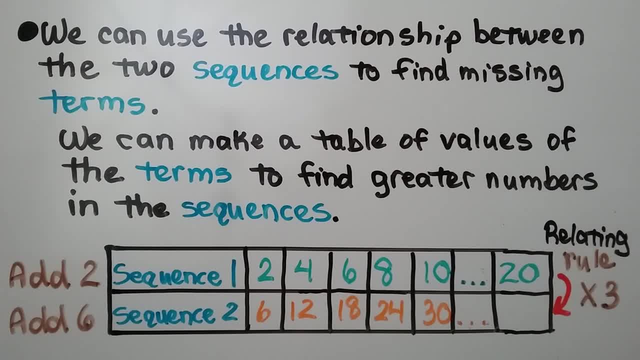 Remember, terms are the numbers that are in a sequence And we can make a table of values of the terms to find greater numbers in the sequences. So when you see this dot dot dot, that's called an ellipsis. It means that we're jumping from 10 to 20.. 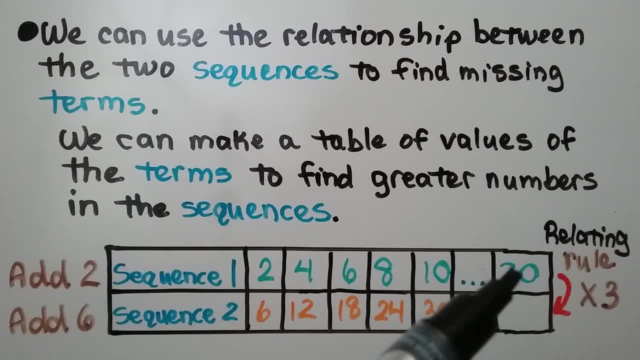 So we're gonna jump from 30 to some greater number that is related to 20.. We know that if we multiply a number, a term from sequence one, by three, we'll get the number, the term for sequence two. That means if we multiply 20 times three. 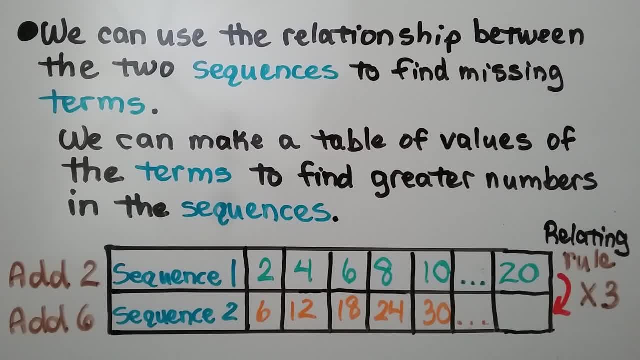 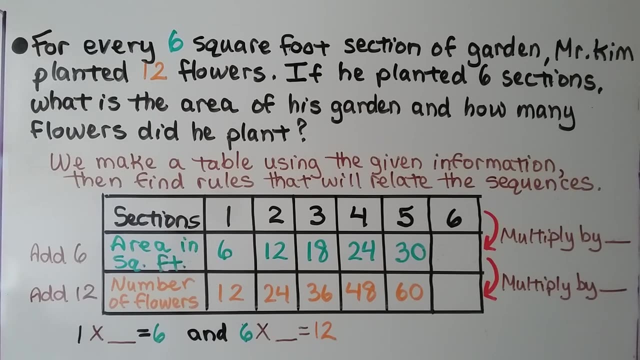 we'll get this unknown term. That would be 60.. Now, if this was very confusing for you, just click the description and go back to video 9.5, and that'll help you out. For every six square foot section of garden, 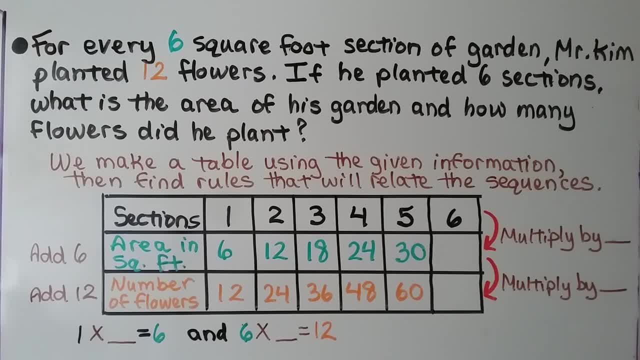 Mr Kim planted 12 flowers. If he planted six sections, what is the area of the garden and how many flowers did he plant? So we can make a table using the given information, then find rules that will relate the sequences. So here we have the sections. 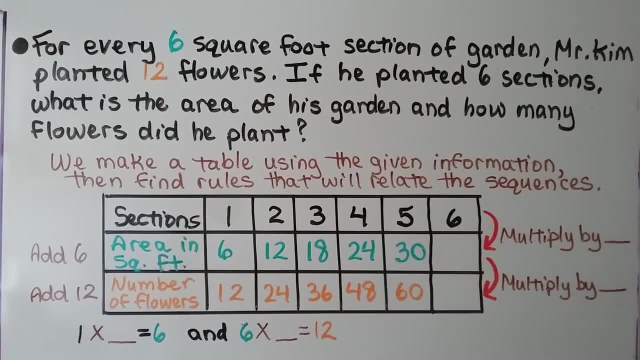 One section, two, three, four, five, six- We're looking for six- And the area in square feet for one section is six square feet, which is 12 flowers. We're going to add six for the area in square feet. 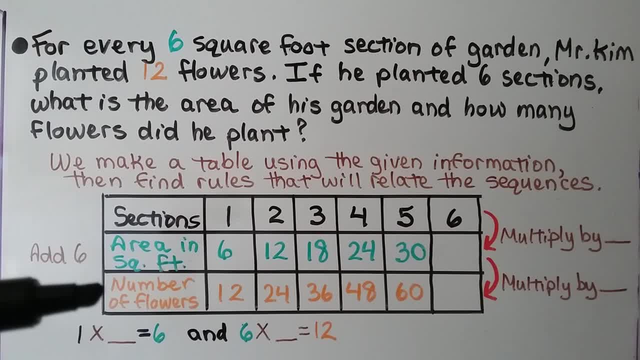 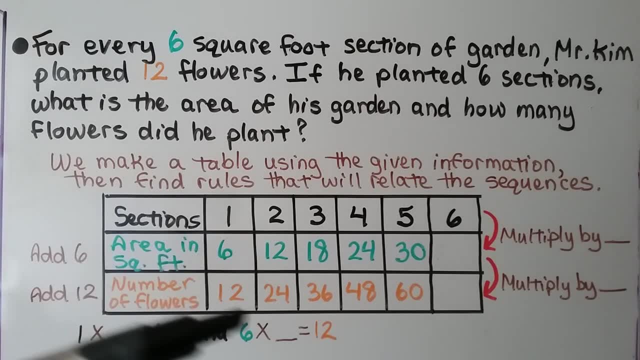 because if he has two he'll have double this, That'll be a 12.. And if the number of flowers for one section is 12,, we're going to add 12 to have 24 for two sections And we can fill in the unknown information in the table. 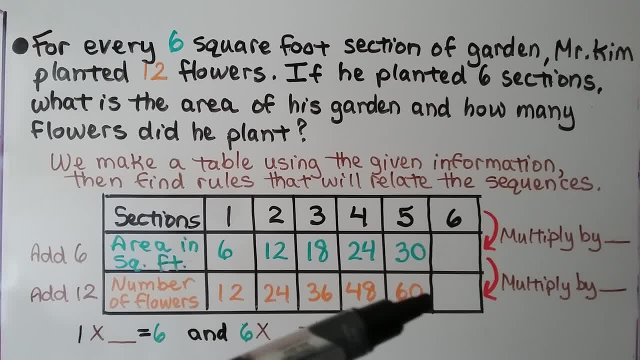 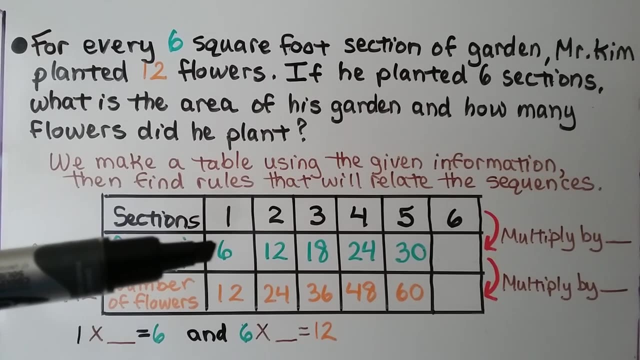 by either adding six for the square feet or adding 12 for the number of flowers. We can also look at the relationship between the sections, the area in square feet and the number of flowers. One to be a six is one times six. 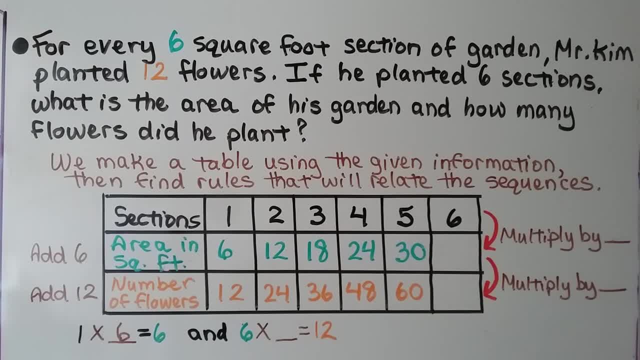 We could do: one times six equals six, And six times two would equal 12.. So we could do times two And we can check for two sections to see if this rule works. Two times six is 12.. Yeah, so times six works here. 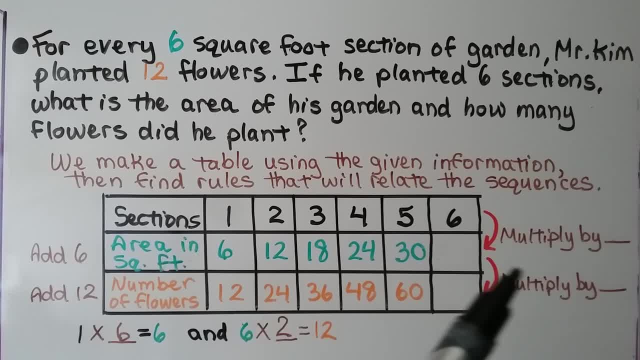 And 12 times six is 12. And 12 times two is 24.. So, yes, so this would be multiplied by six and this would be multiplied by two. Now we can find the missing information for six sections. It would be six times six, which would be 36.. 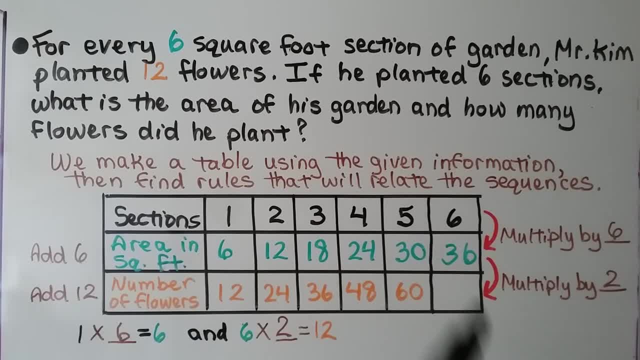 And remember, we also could have just done 30 and added six, And for number of flowers we do 36 times two, or we could even do 60 plus 12.. So that's it for number of flowers, 12.. That would be 72.. So the area of his garden would be 36 square feet and he would have 72 flowers. 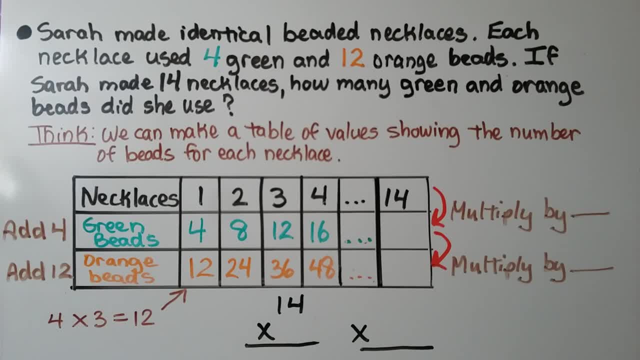 Sarah made identical beaded necklaces. Each necklace used four green and 12 orange beads. If Sarah made 14 necklaces, how many green and orange beads did she use? So we think we can make a table of values showing the number of beads for each necklace. 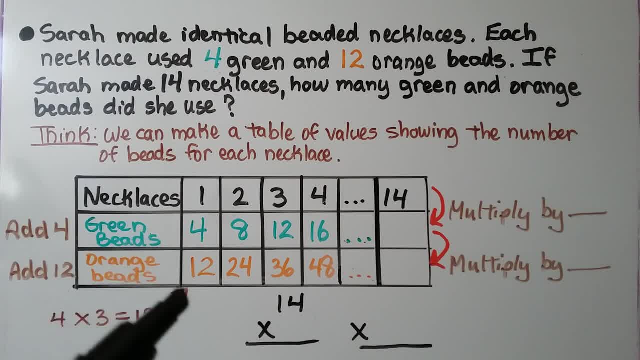 If she makes one necklace, she's going to use four green beads and 12 orange beads. If she makes two necklaces, then she would use eight green beads and 24 orange beads, And the rule for this sequence for green beads is to add 4.. And the rule for the orange beads is to add 12.. But what about 14.? 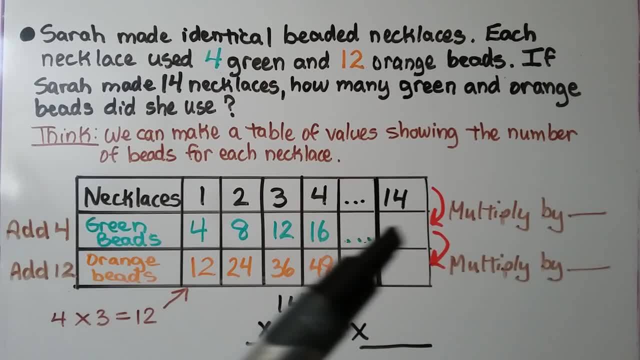 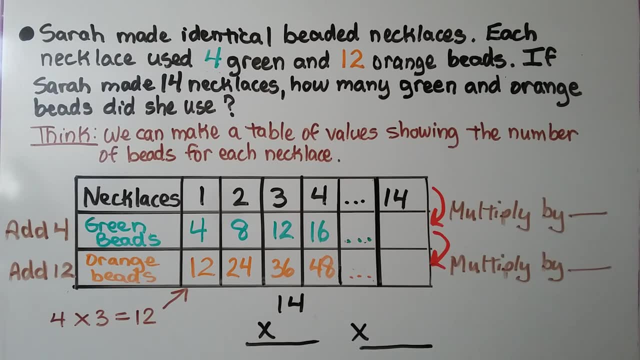 We could make a video about making 12. long table: adding 4 and adding 12, making the table keep going until we got to 14. or we could find a rule that we can multiply the necklaces by to get the green beads and to multiply the green beads by to get the orange beads when we 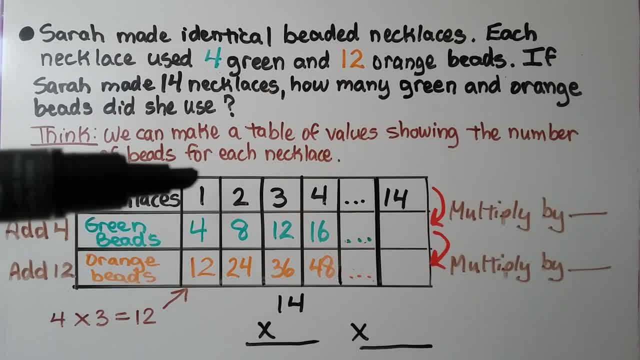 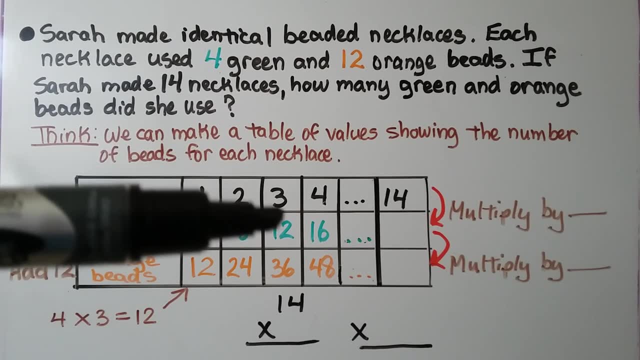 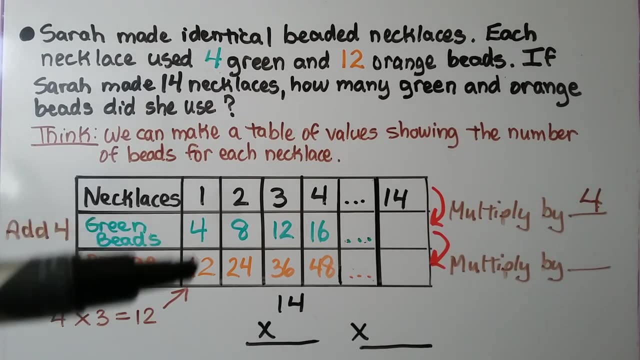 look at the values that we have we have: 1 times 4 is 4. 2 times 4 is 8. 3 times 4 is 12. so the rule here is: multiply by 4. from the green beads to the orange beads. we're multiplying by 3. 4 times 3 is 12. we check it with this one: 8 times 3 is 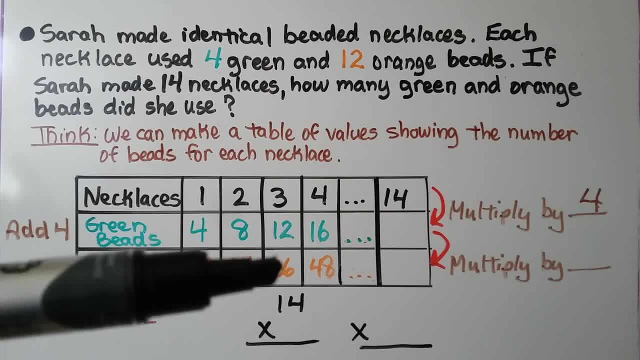 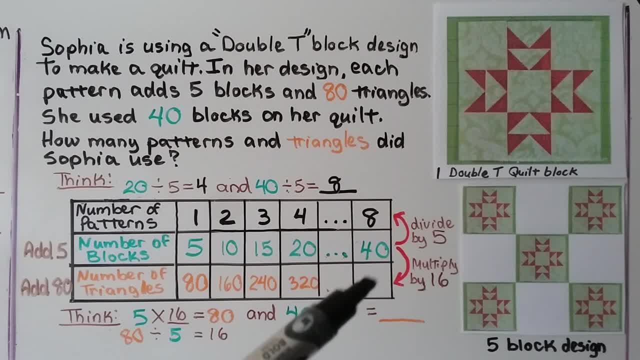 multiply 14 by 3, that means to find the green beads for 14. we need to multiply 14 by 3. that means to find the green beads for 14. we need to 16 to find the number of triangles. We do our multiplication and we find it's 640 triangles. 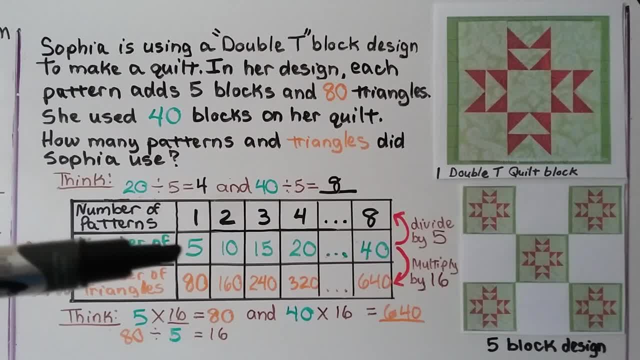 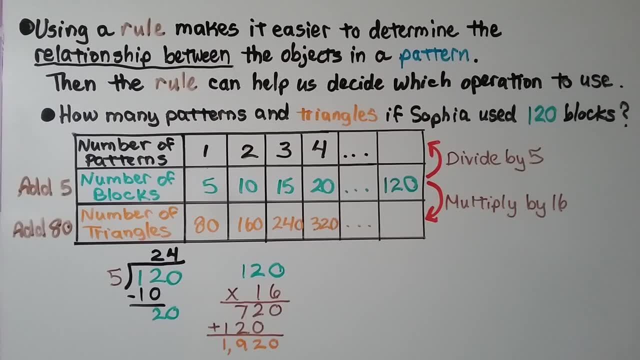 We needed to use the given information- the number of blocks- to compare it to the number of patterns and the number of triangles. Using a rule makes it easier to determine the relationship between the objects in a pattern. Then the rule can help us decide. 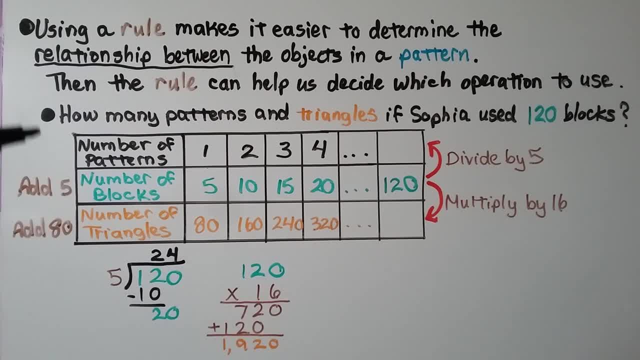 which operation to use How many patterns and triangles. if Sophia used 120 blocks in her quilt, We can use the same rule: divide by 5 and multiply by 16, to find the number of patterns and the number of triangles. 120 divided by 5 is 24.. We put a 24 for the number. 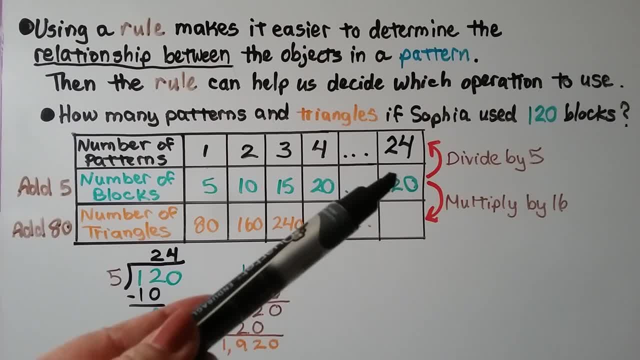 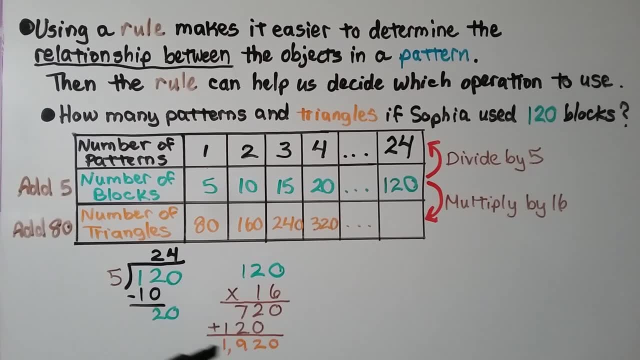 of patterns. The rule from the number of blocks to the number of triangles was multiplied by 4.. We multiply by 16, so we can multiply 120 times 16. We get 1920. That's a lot of triangles. So we know, if she uses 120 quilt blocks she's going to need 1920 triangles and she won't. 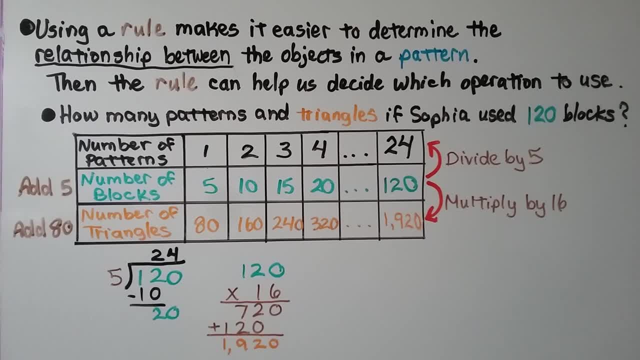 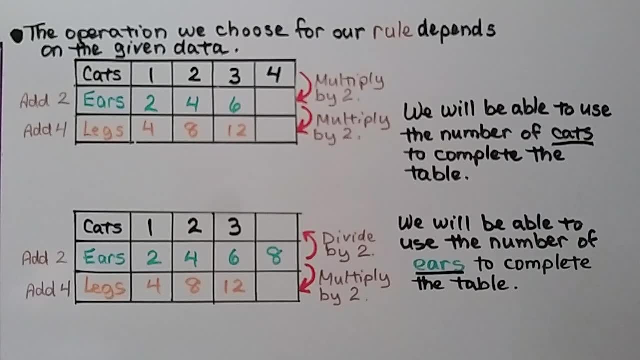 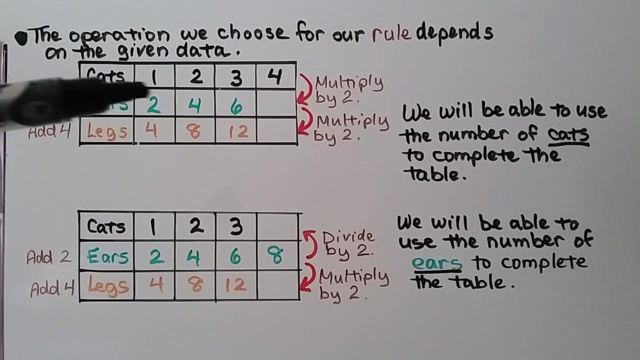 be able to make 24 patterns. The operation we choose for our rule depends on the given number of blocks. If we have a cat, it has two ears and four legs. If we have two cats, it will have four ears and eight legs. For this sequence, we add two because there are 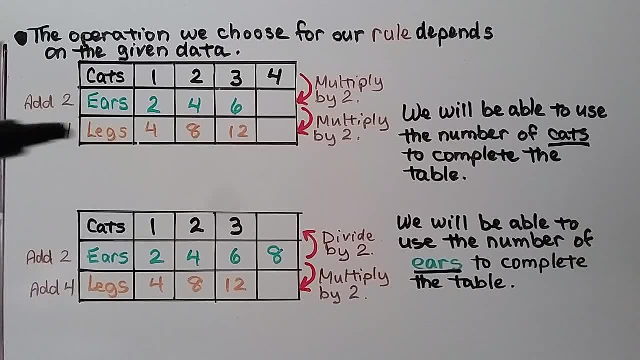 two ears on each cat. For this sequence of legs, we add four, because there are four legs on each cat. To go from cats to ears, we multiply by two. To go from ears to legs, we multiply by two And we'll be able to use the number of cats to complete the table For multiplying by. 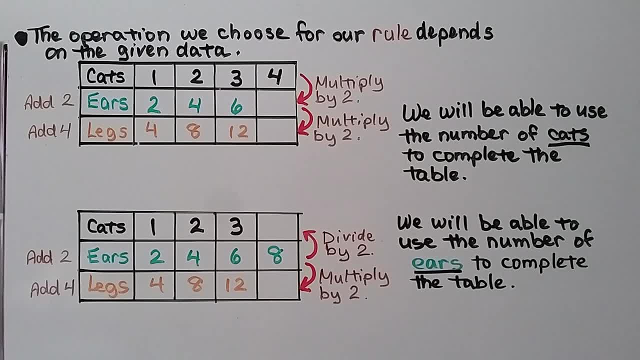 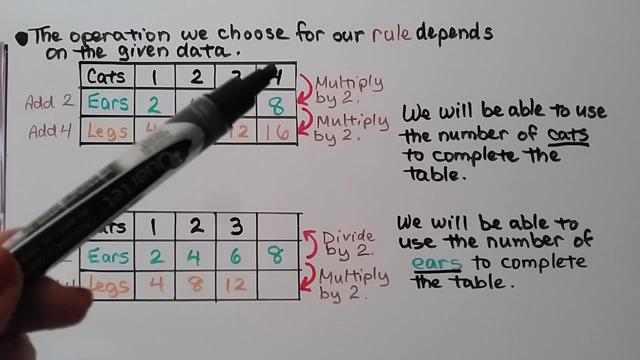 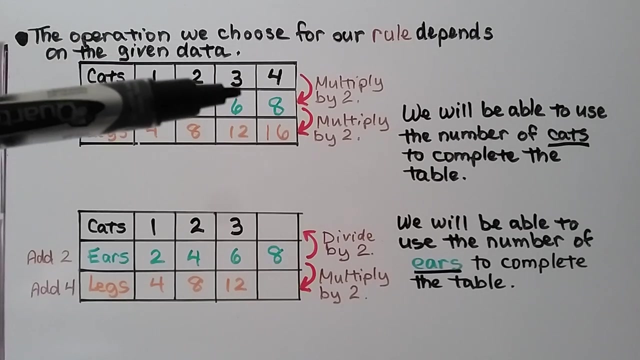 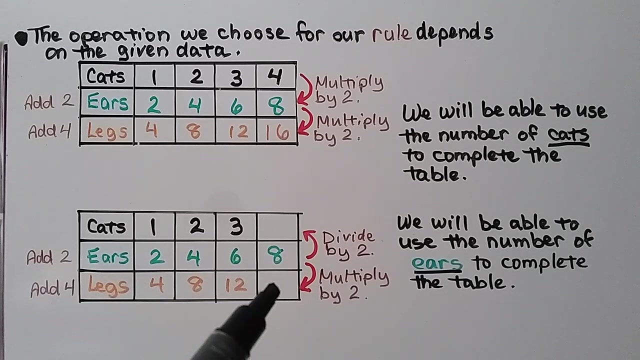 two, four cats times two would be eight ears. Eight ears times two would be 16 legs. Because the information we were given was four cats. we used the four to help us find the other missing values. Here we have the number of ears, but we don't have the number of cats, and we don't have 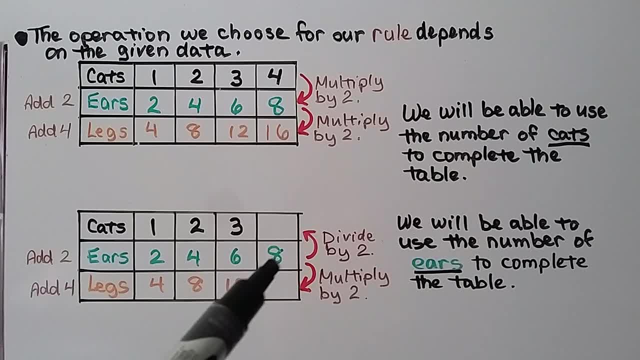 the number of legs, We'll be able to use the number of ears to complete the table. We'll look at the relationship for six and three. Six divided by two is equal to three. Four divided by two is equal to two, So that means we'll do eight divided by two, which 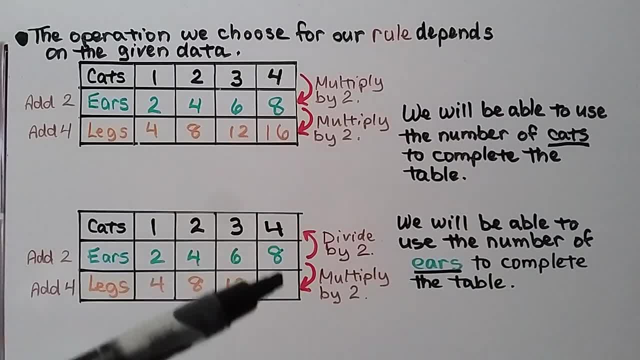 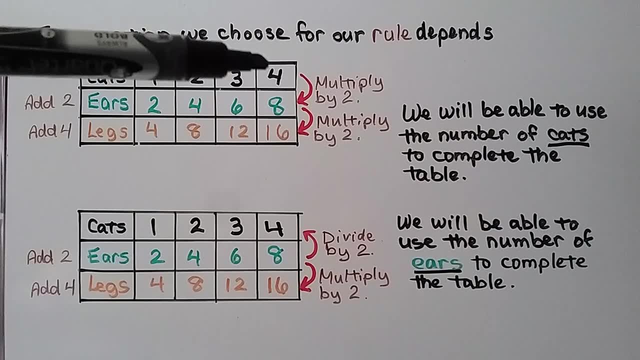 is a four, Then we can do 8 times 2,, which is 16.. Because we were given the number of cats in this table, we were able to come down with our arrow and multiply by 2, then come down again and multiply by 2.. 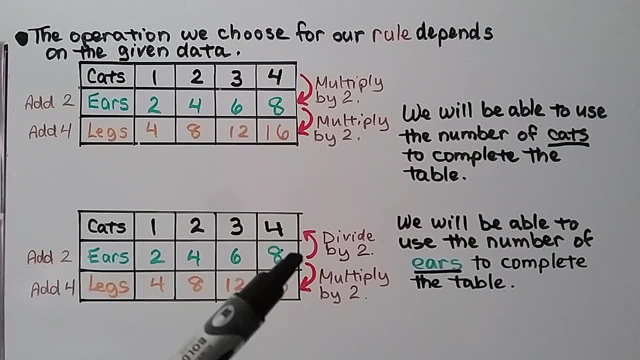 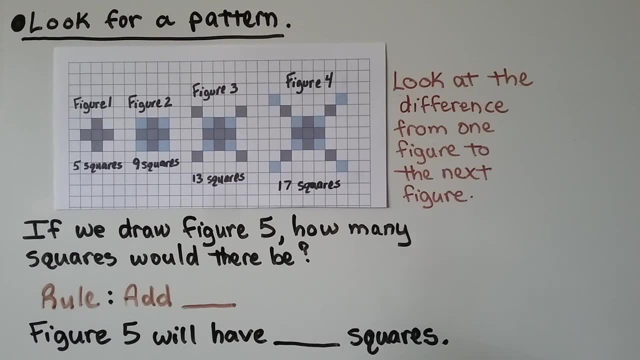 Because in this table we were only given the number of ears. we had to go up and divide by 2 and go down and multiply by 2.. So the operation we choose for our rule depends on the given data. We need to look for a pattern. 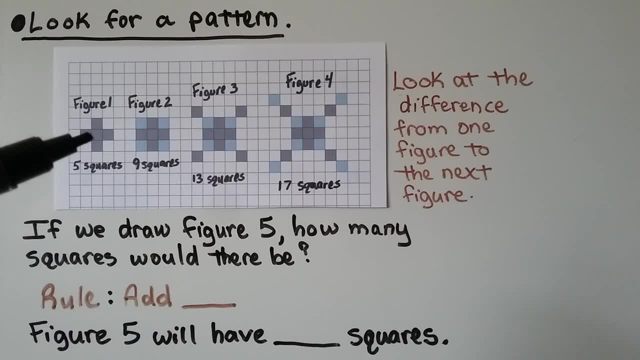 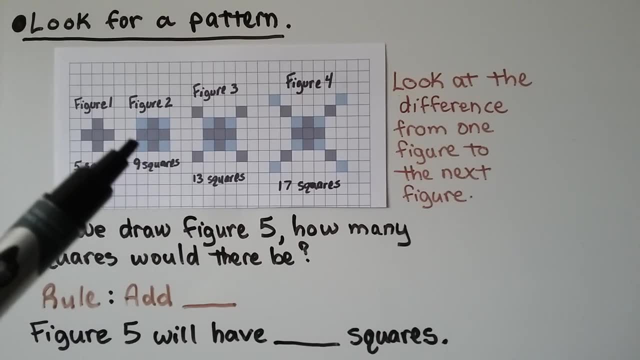 Look at Figure 1.. There are 5 gray squares. Now in Figure 2, there's 5 gray squares and in each corner there's a blue square, so there's now 9 squares. For Figure 3, we have the same pattern as Figure 2, but now we've got a gray square. 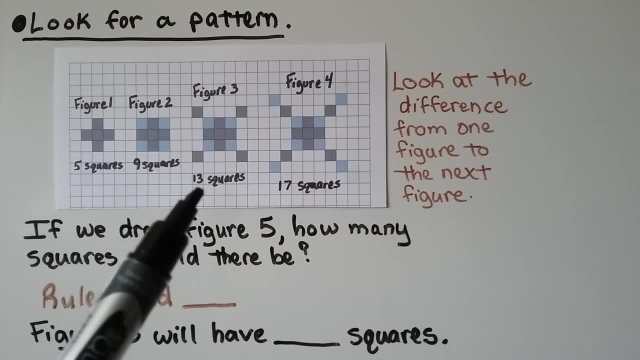 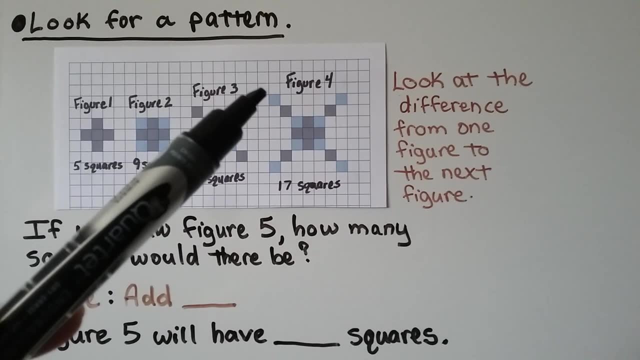 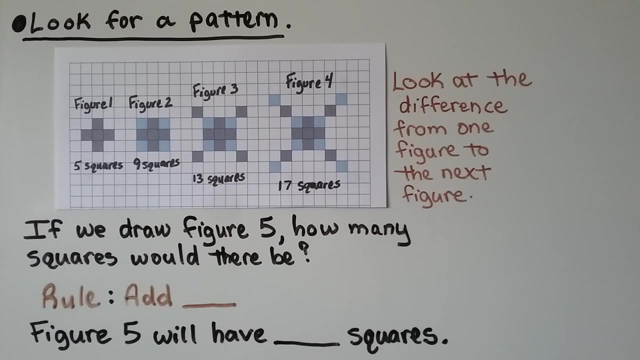 in each corner There's 13 squares in all. For Figure 4, we have the same pattern As Figure 1,, 2, and 3, but now we've got light blue squares in the corners. Now there's 17 squares.